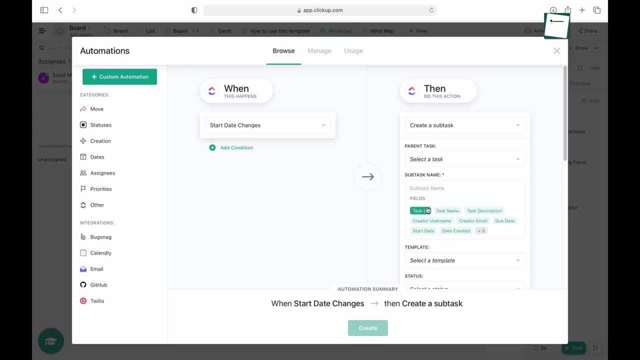 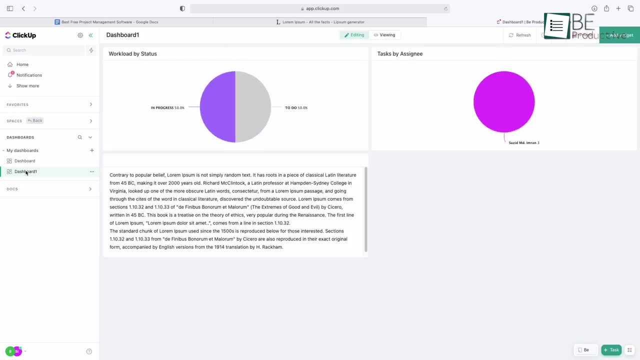 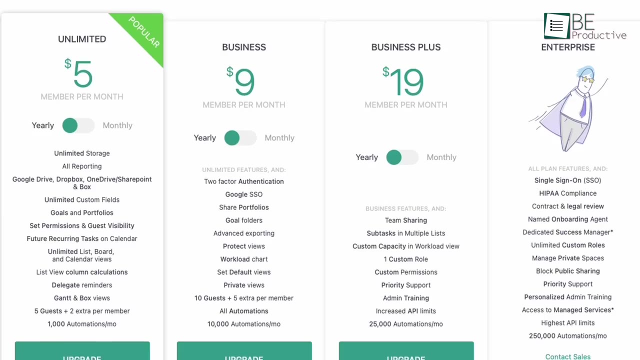 functionalities. You can save time with task automation, add custom fields and so on. With dashboards, you can add visual widgets for team members, time tracking, tasks, docs and many more into one single place. There are four other premium plans as well. Keep in mind that the onboarding process isn't 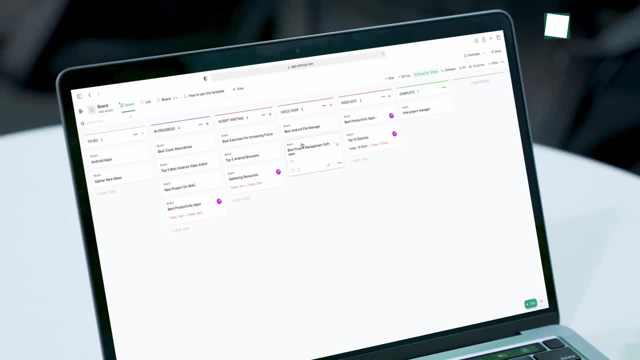 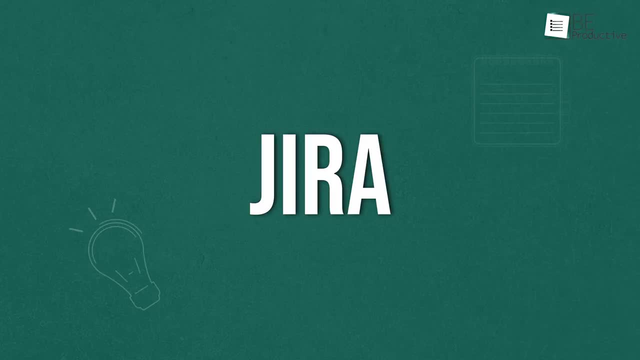 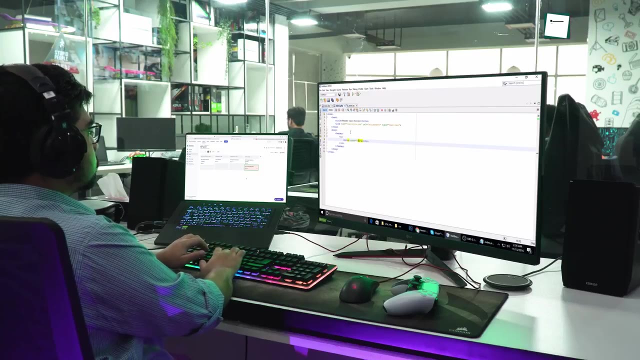 as simple as some other project management like Trello, But considering the extra features that are also completely free, ClickUp is really worth trying. Jira is yet another project management app that is built specially for every member of your software team to plan, track and release great software When you first sign up for. 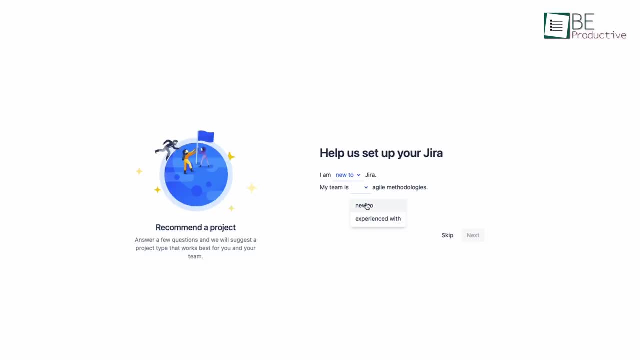 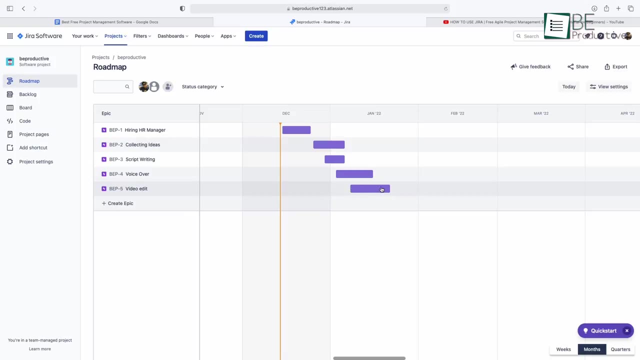 ClickUp, you'll see a list of the best free project management software that you can use. It'll ask you a few questions about your project level of experience and other methodologies and then recommend a project template for you. For scrum projects, you have to add epics to the roadmap page, which you'll find on. 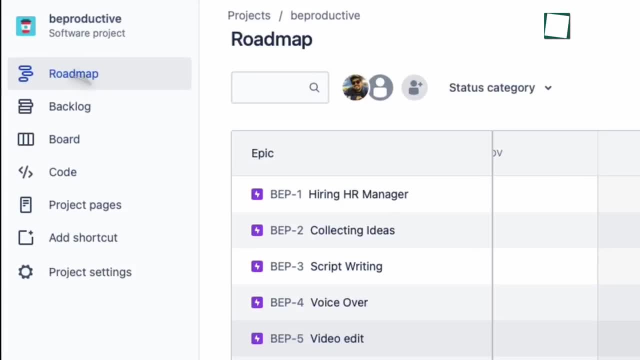 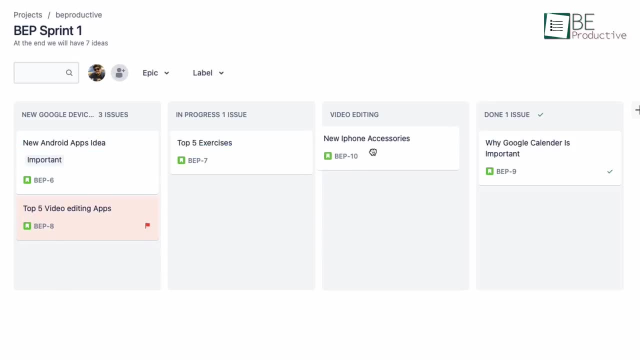 the left side of the screen. Beneath it you have the backlog where you can add issues and fill details to your project and assign them to sprints. Inside the board you can create a to-do list, move them into progress and then done when you finish a project In. 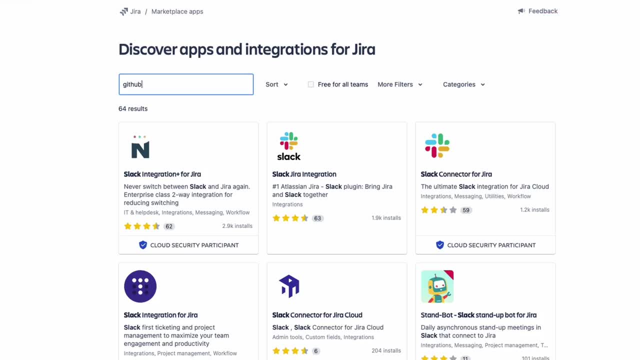 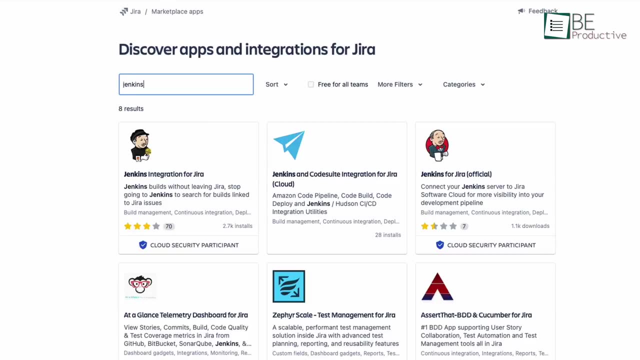 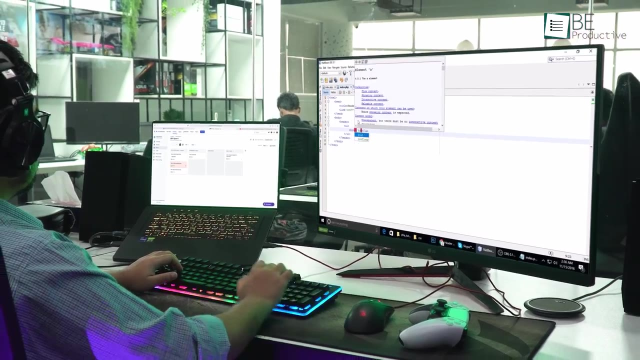 the project pages, you can choose to idiots different templates. this project management app also integrates well with other development tools like github, sentry and jenkins to update and track your backlog. finally, this app is available for web android as well as ios devices, so if you're looking for a project management app for 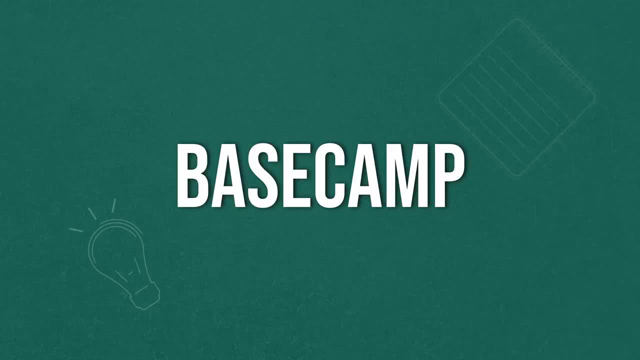 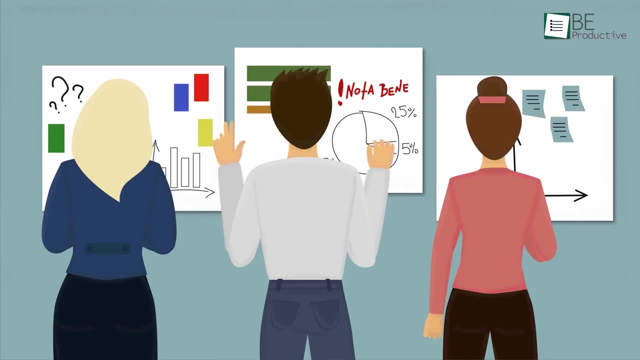 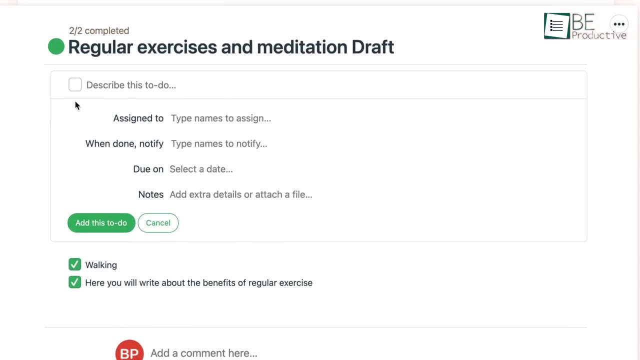 software development. we highly recommend this one. when you're working with your team, it's important to bring all the ideas together, and the base camp exactly does that by helping you organize all your projects in one place and split work between teams. with this app, you can create to do's to assign. 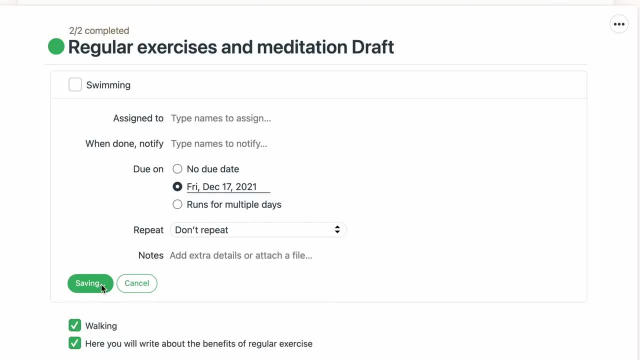 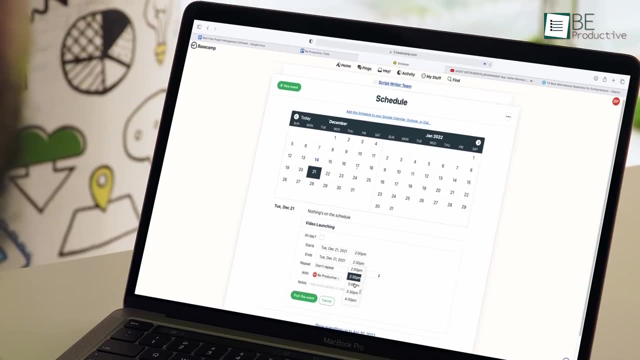 items to your team members and due dates for your projects. it also has a message board that can be used to communicate with teammates for receiving project updates and feedback. another feature that comes in handy is the schedule manager to automate setting up meetings and subscribing to an event. 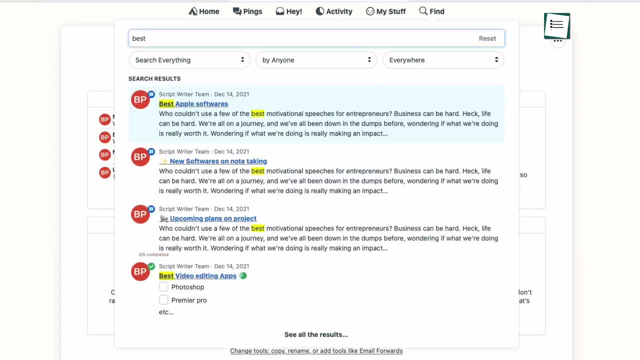 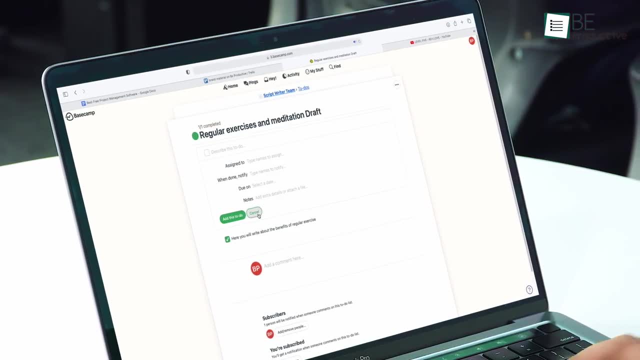 you can also use the search button at the top to quickly find something that you're looking for. there are also options for direct messaging, show notification and activities. the free version is great for personal projects and light use, but you can upgrade to the business plan of base camp to. 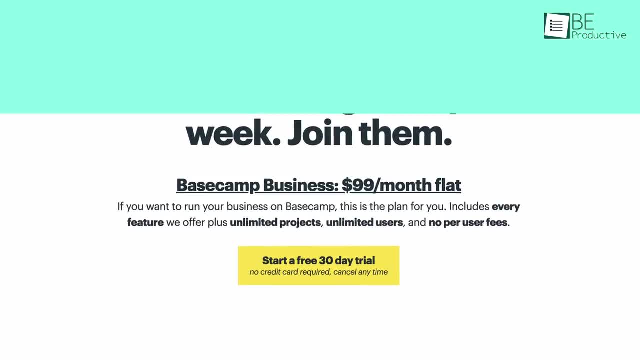 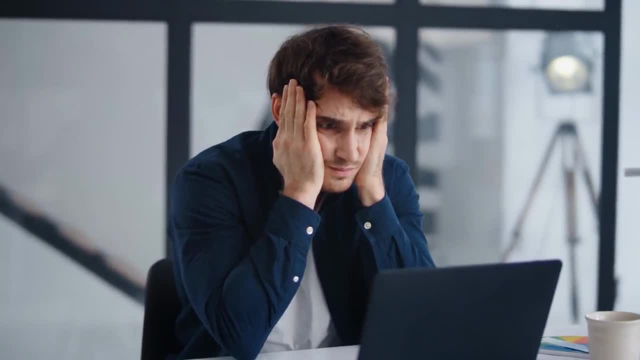 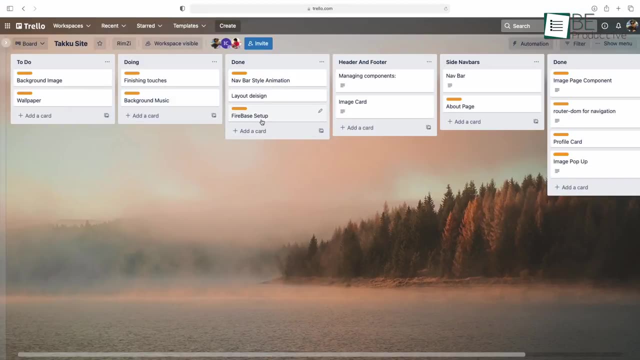 unlock every feature that is suitable for large businesses. the problem with most project management tools is they aren't just easy to use, but trello is different. it's a kanban style app that helps you organize projects with an easy to use layout. because of that, you can easily hit the ground without spending hours of training. 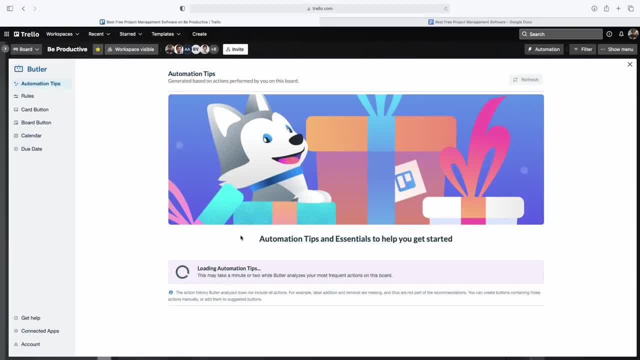 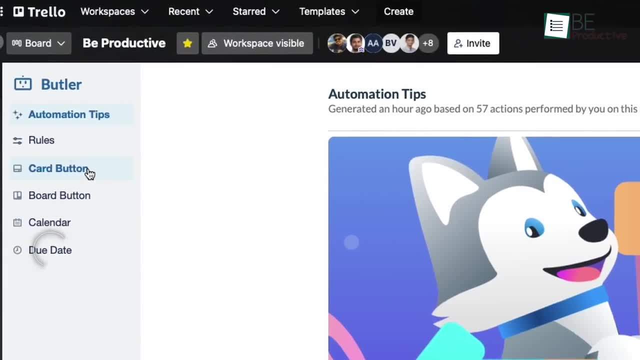 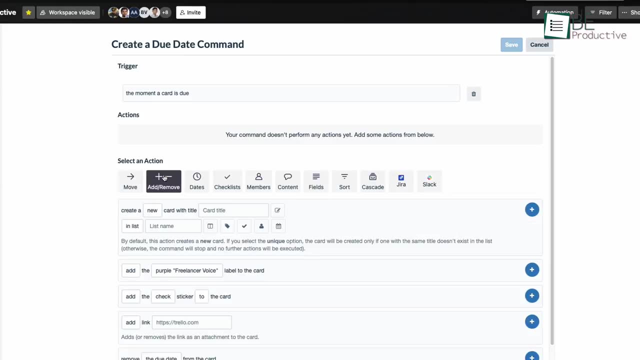 it stands out from other workflow management tools due to a few smart features, like butler, an automation tool that lets you automate several commands, including card board and due date. this automation saves you from having to click and drag cards around so much, but it also helps workflows and processes run like clockwork to prevent mistakes. 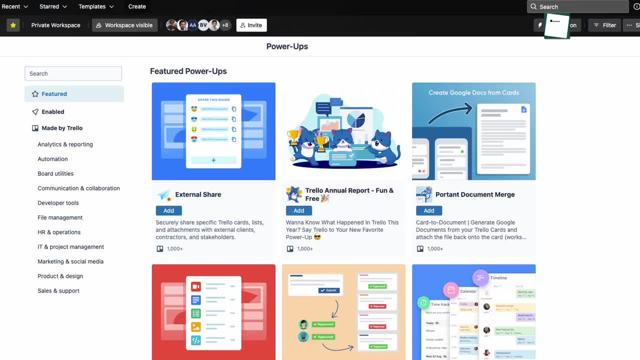 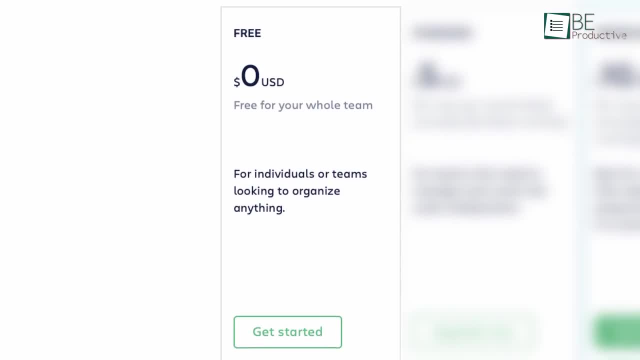 furthermore, trello's power-ups are now unlimited for every user in trello. this means you can do endless customization to your boards, cards and views. it offers a free plan with basic features, but if you need even more functionalities, you can choose one of the three paid plans. 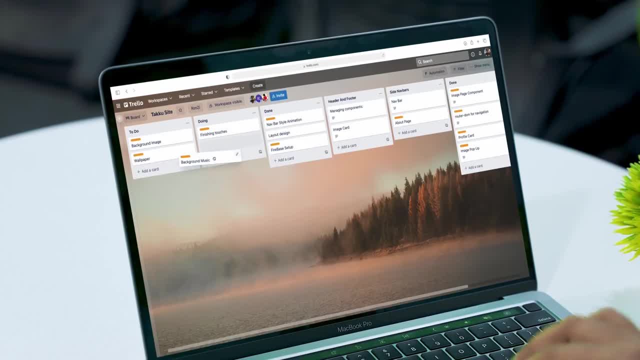 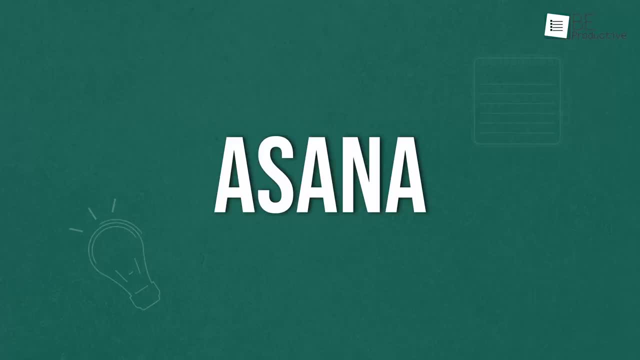 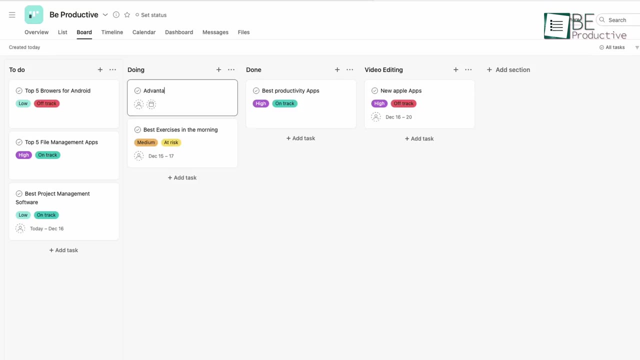 including standard, premium and enterprise. all in all, if you want a simple project management app without any learning steps, trello is an excellent choice for you. last on our list is asana, a great alternative to trello, which is also simple to use, but also easy to use and can be used for a lot of projects. 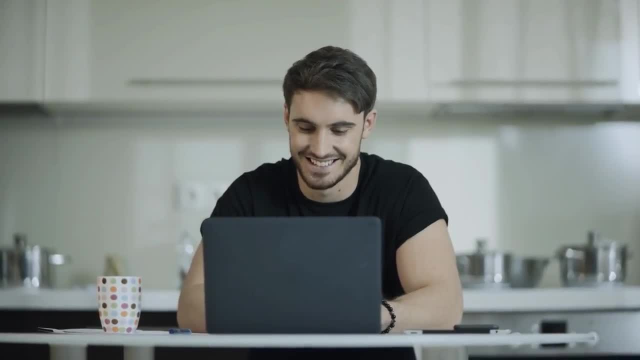 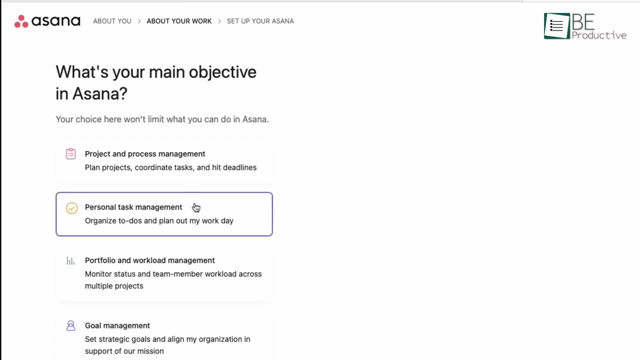 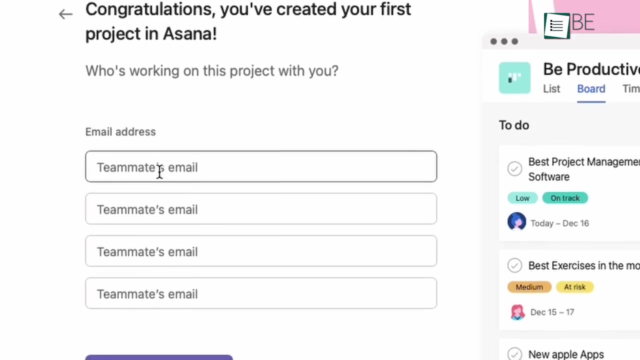 perfect for people who are looking for some extras in their project management software. when signing in for the first time, it will ask you some questions like what type of work you're into and what project you and your team are doing. after finishing signing up, you'll be left on the main home screen of the app, where the first thing you want to do is: 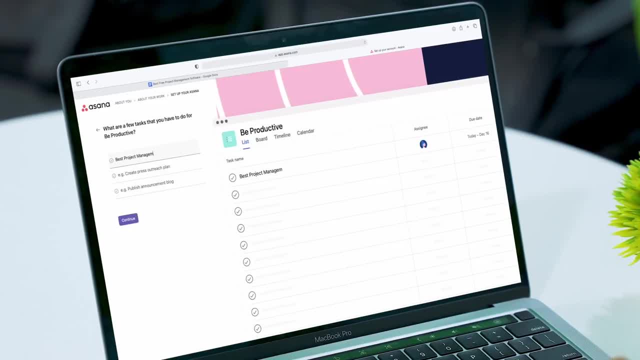 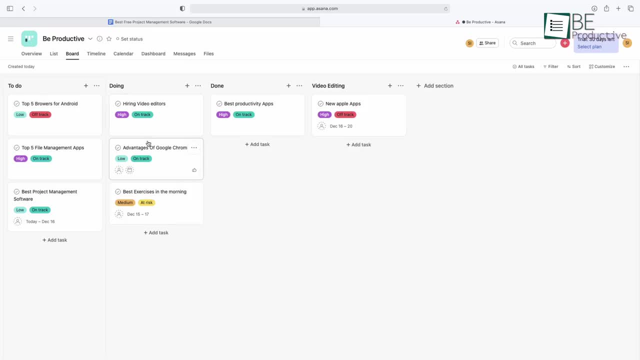 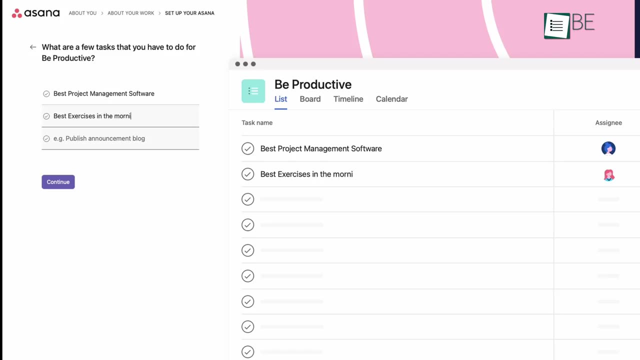 to invite people to your projects. after that you can add tasks to your project, set due dates, add descriptions and much more. you can move the card from doing to done if the task just like you do in trello. for added bonus, you can change the layout to list board timeline and.